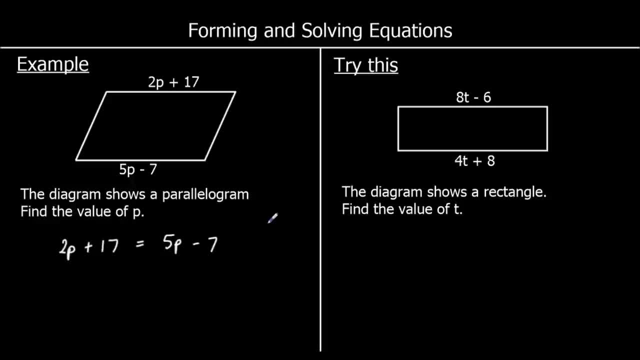 The opposite sides of a parallelogram are equal, So the expression for one of them must be equal to the expression for the other one. So we've formed the equation. Now we solve it. We have p's on both sides of the equation. 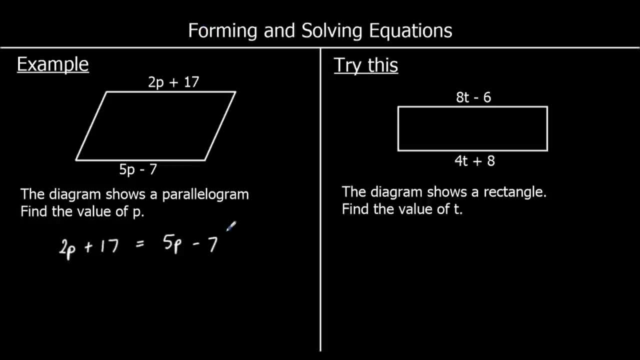 and we are going to get rid of the smallest one first. So that's 2p. So we're going to take 2p away from both sides, which leaves us with 17.. 17 is equal to 3p, 5p. take away 2p is 3p minus 7.. We want p by itself, So we're going. 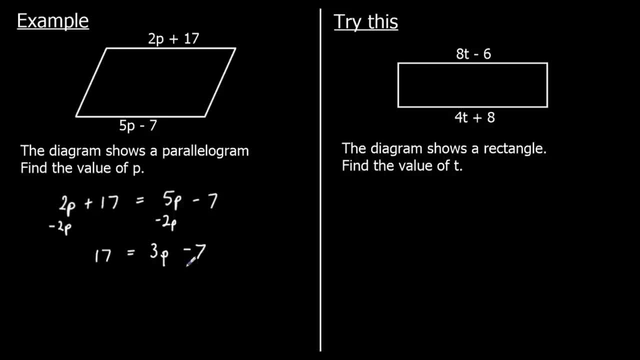 to get rid of minus 7 by plusing 7 to both sides. So 17 plus 7 is 24 and that's equal to 3p. We have 3 times p at the moment. Now let's think about this: shall we To get rid of the 3,? we do the opposite. 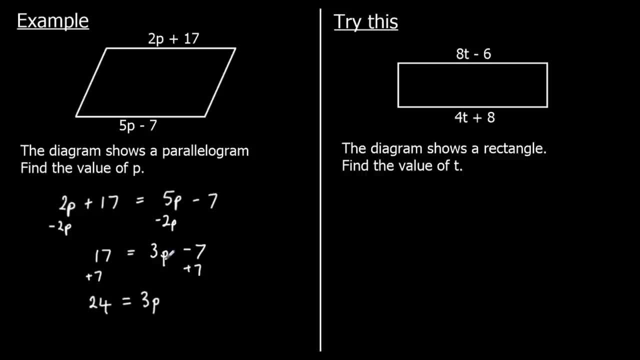 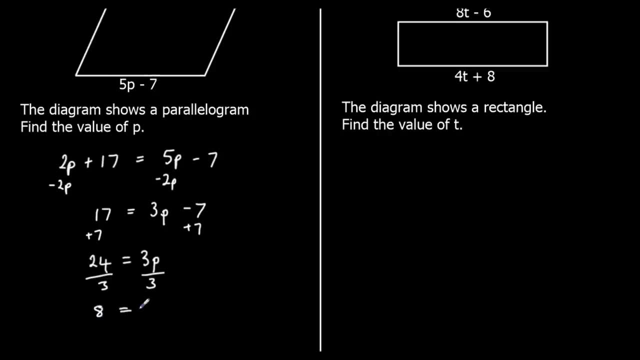 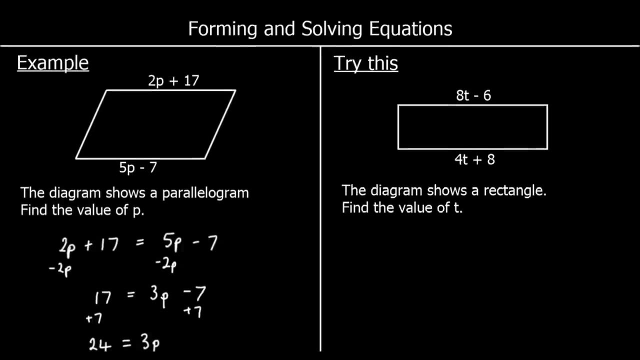 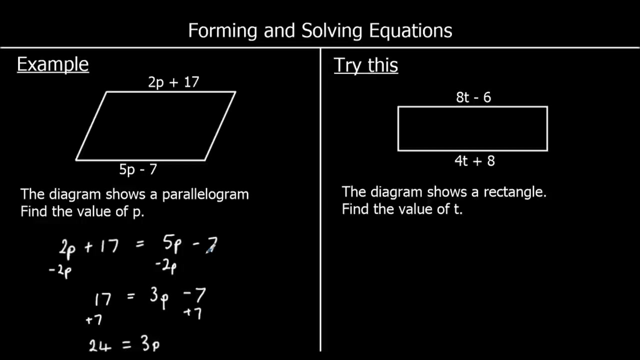 of times by 3, which is divide by 3.. So divide both sides by 3.. So we get 8 equals p, or p equals 8.. Okay, a question for you to try. So pause the video and give this one a go. 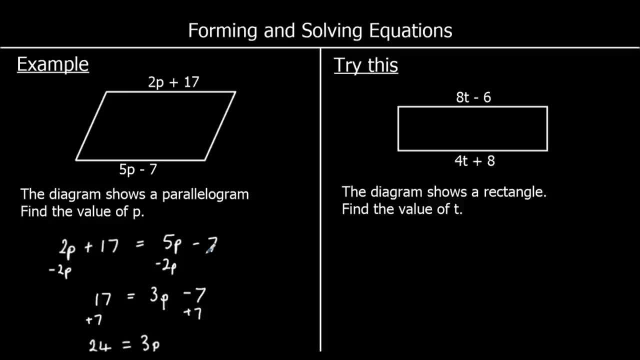 we need to know. the opposite sides of a rectangle are equal, So 8t minus 6 must be equal to 4t plus 8.. We're going to get rid of the smallest t first, which is 40. So take 4t away from both sides. 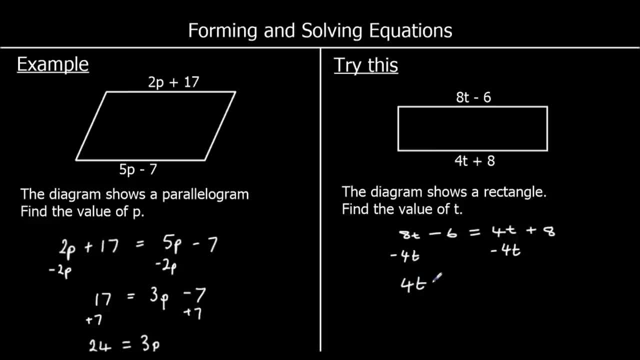 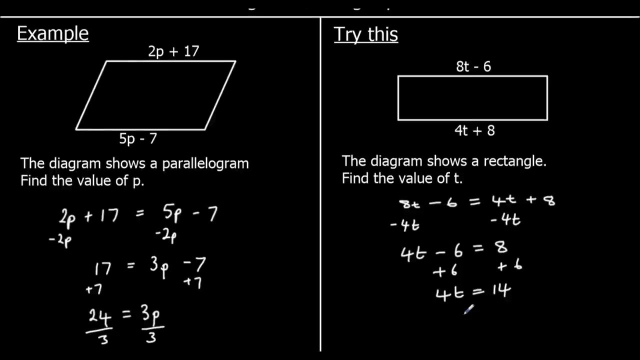 So we have 4t minus 6 equals 8.. We want t by itself. We're going to get rid of minus 6 by plussing 6 to both sides. So we have 4t equals 14. And we divide both sides by 4 to get t by itself. 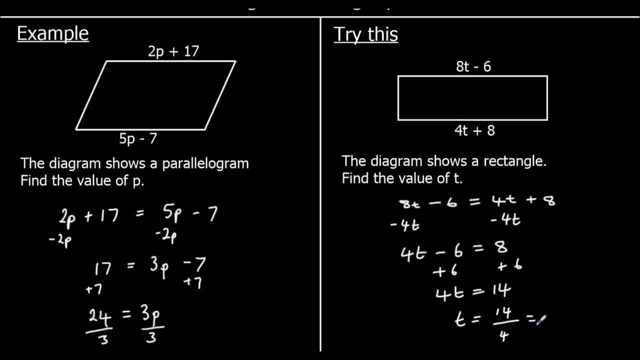 So t is 14 over 4.. They're both even so we can half them, So that's 7 over 2.. 7 over 2 is the answer. If you wanted to write it as a decimal, you could. 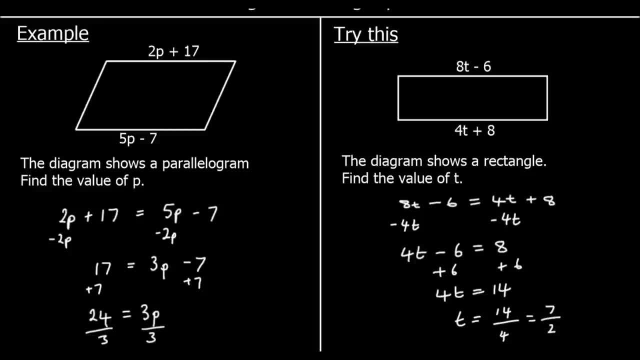 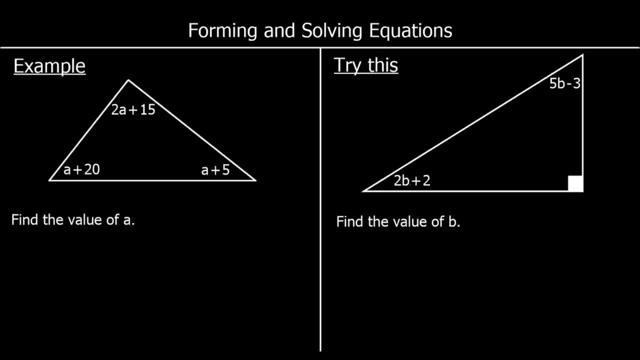 And that would be 3.5.. So we have a different example here This time. what we need to know is that all of the angles in a triangle add up to 180 degrees. We can assume that all of these expressions are in degrees. 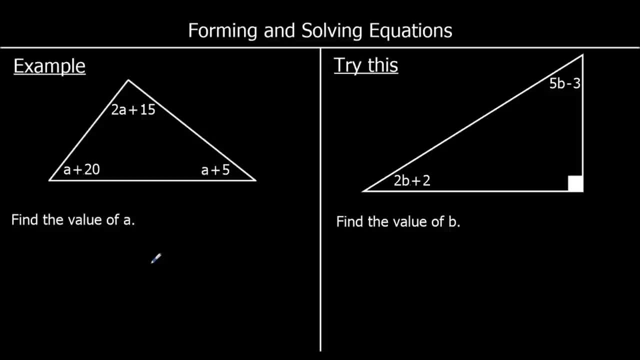 So we can make an equation. We can form an equation by adding all of these up and making it equal to 180.. So we can say a plus 20 plus 2a plus 15 plus a plus 5. Is equal to 180. 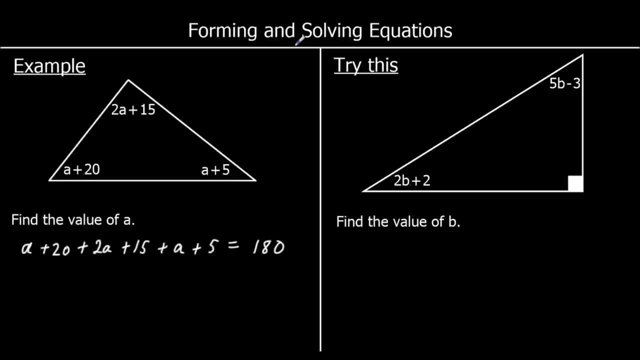 And again we can assume it's all in degrees. We can simplify this. We've got a terms: a plus 2a plus a, That's 4a, And 20 plus 15 plus 5. That's 40.. 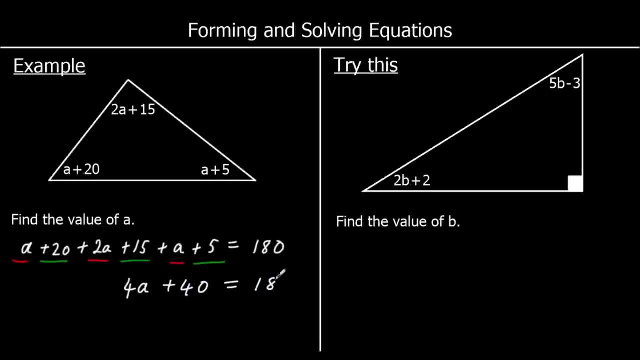 So 4a plus 40 equals 180.. And again, we can assume that all of these are in degrees. So 4a plus 40 equals 180.. We want to find out what a is. So let's take 40 away from both sides. 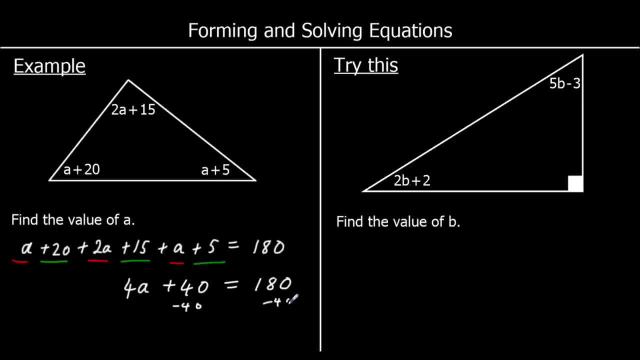 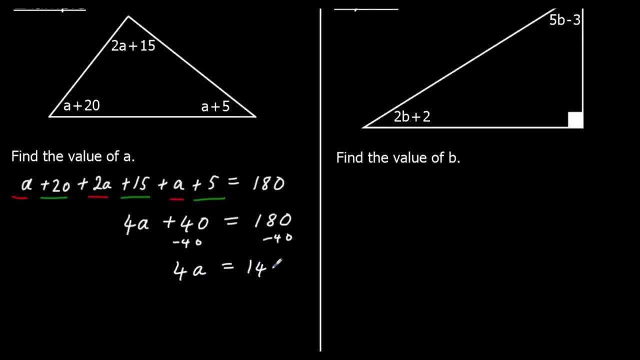 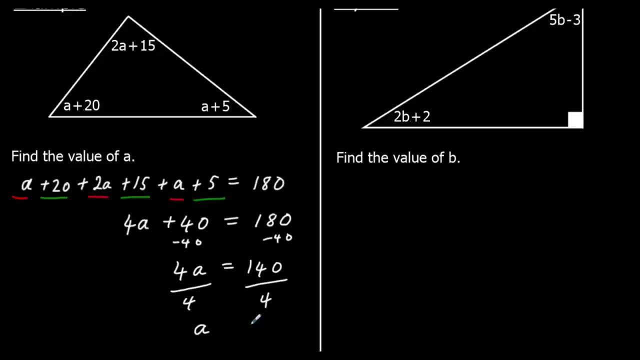 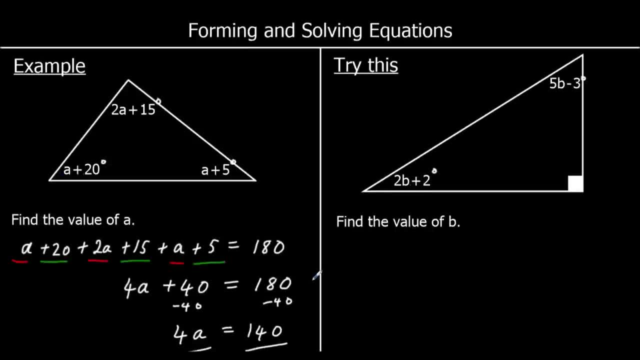 you to try. So pause the video and have a go at this one. The angles in a triangle add up to 180 degrees, So we can say that all of these angles added up makes 180.. So 2b plus 2 plus 5b minus 3 plus. 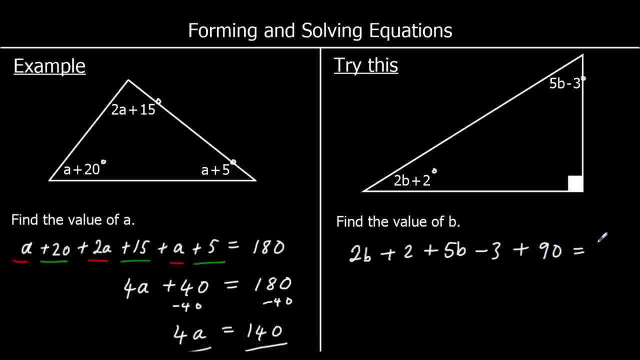 a 90 degree angle is equal to 180. And what we could actually do if we could imagine take 90 off of both sides. we can say: 2b plus 2 plus 5b minus 3 must equal 90. So we've already got a 90 degree angle: 180. take away 90 is. 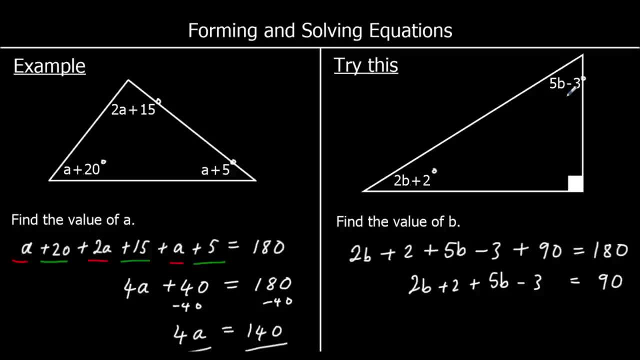 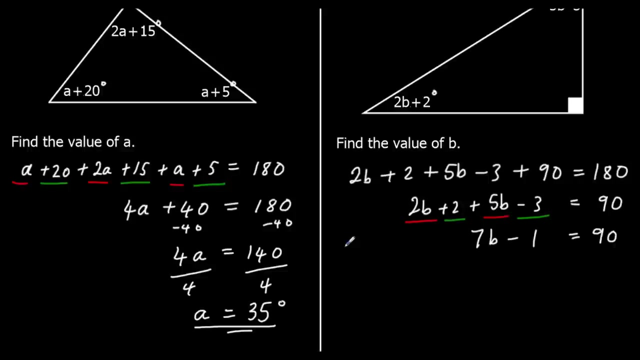 90.. two angles must add up to 90 and we can collect the like terms. 2b and 5b is 7b, and 2- take away 3, is a negative 1. so 7b minus 1 is 90. we want 7b by itself. so 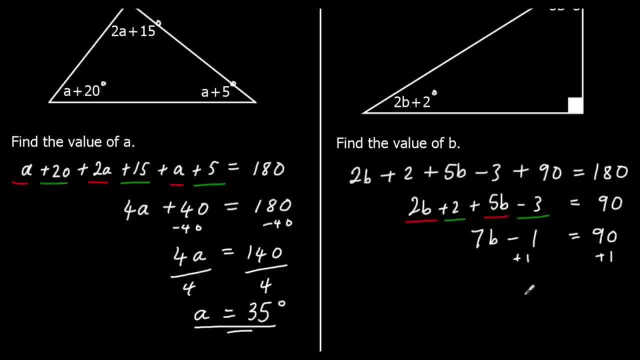 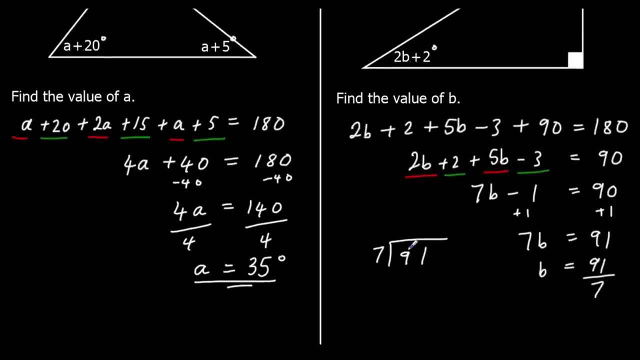 plus 1 to both sides. so 7b is equal to 91. so B divide both sides by 7. so B is 91 over 7. how many sevens go into 91 there oneself and goes into nine? there are two left over and 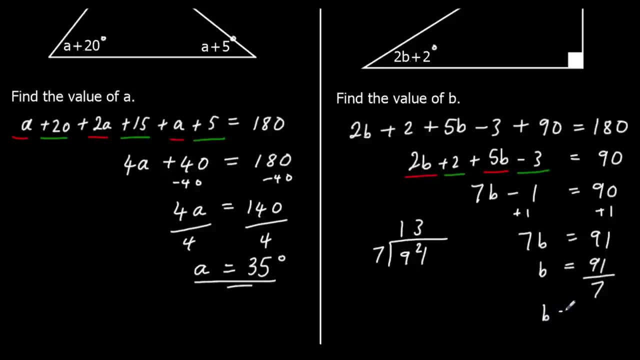 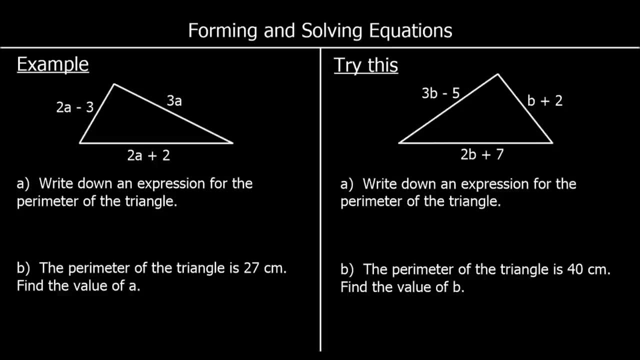 B7's going to 21.. So B is 13.. And again I'll write degrees And the next example. So we've got a triangle. again We have expressions for the lengths of each of the sides of the triangle And the question says, part A: write down an expression for the perimeter of the triangle. 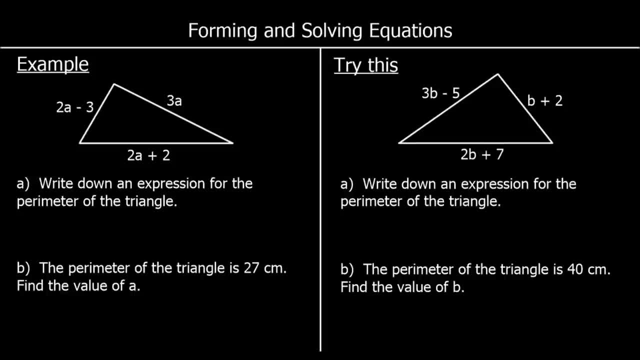 So perimeter is all of the lengths, all of the sides added up. So that's going to be 2A minus 3 plus 3A plus 2A plus 2.. And we'll collect like terms. We've got the A terms. 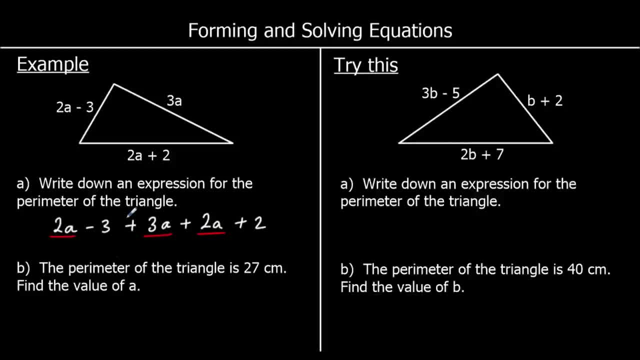 2A plus 3A plus 2A, which is 7A, And we have. We have 2. take away 3, which is minus 1.. So our perimeter is 7A minus 1.. Part B says the perimeter of the triangle is 27 centimetres. 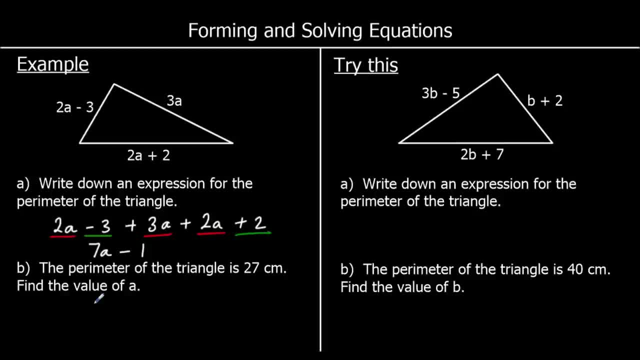 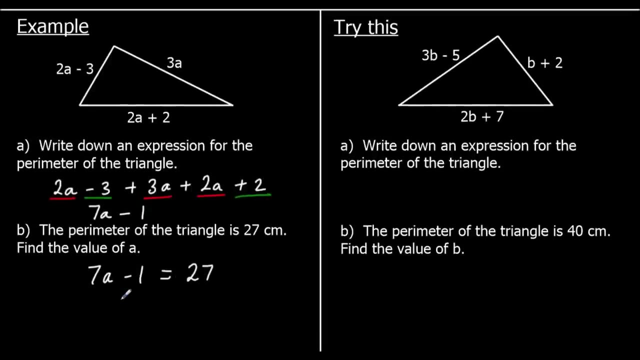 Find the value of A. So we have 7A minus 1 is our perimeter, And that's equal to 27.. So the perimeter is 27.. That means it's equal to 27.. So let's solve this: Plus 1 to both sides. 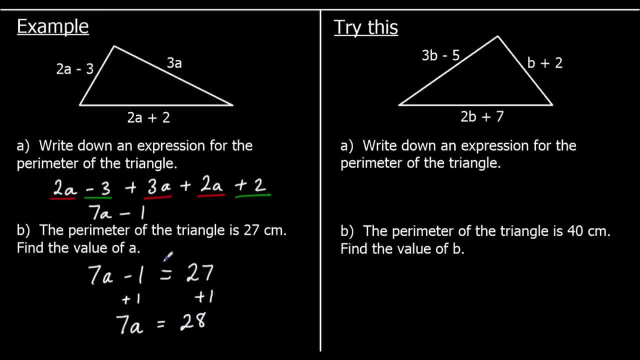 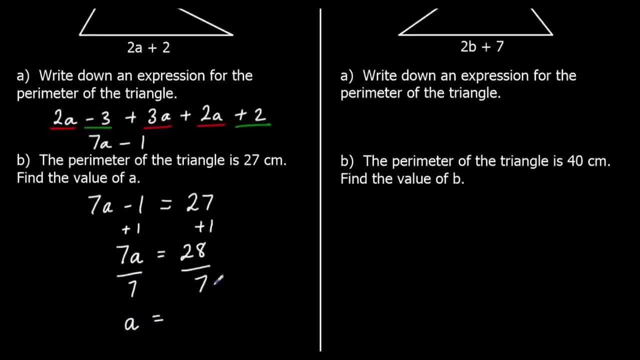 Which gives us 7A equals 28.. We divide both sides by 7. So A is 28 over 7., Which is 4. And it's in centimetres, So I'll write centimetres, So it's in centimetres. 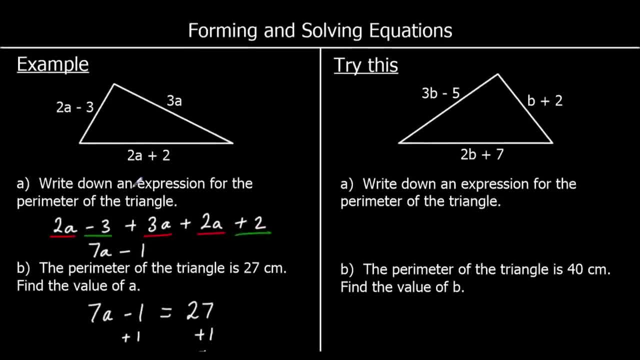 And I'll write centimetres. OK, Question for you to try. So pause the video and give this one a go. So, part A: Write down an expression for the perimeter. So again, that's all of the sides, All of the lengths of the sides added up. 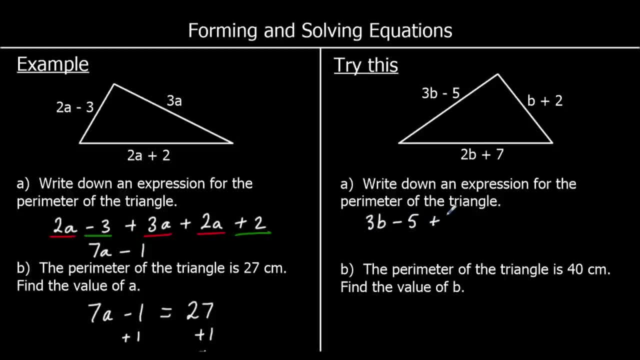 So we've got 3B minus 5.. Plus B plus 2.. Plus 2B Plus 2B plus seven. so collecting the like terms, three b plus another b plus another two b, three plus one plus two, that's six b's. so i've got six b's. 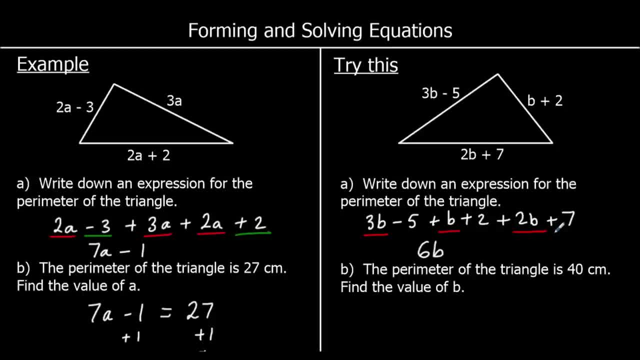 and we have seven plus two, which is nine. take away five, which is four, so six b plus four, and for part b the perimeter is 40 centimeters. find the value of b. so 6b plus 4 is the perimeter and that is equal to 40.. so 6b. 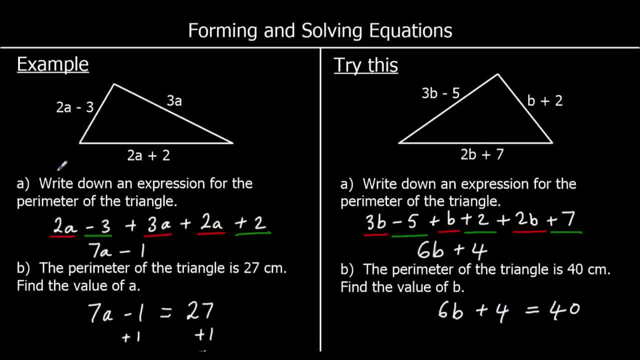 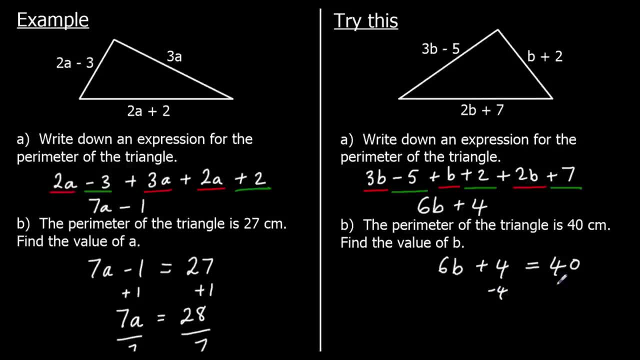 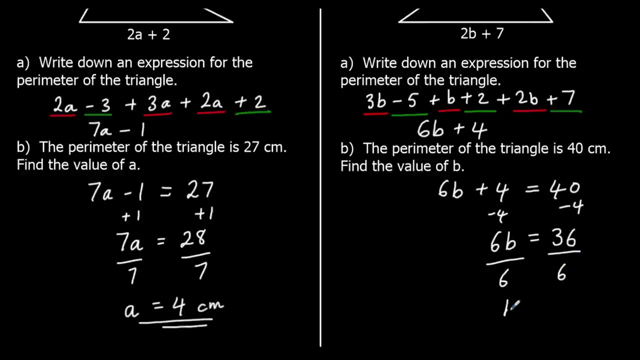 plus 4 is equal to 40.. let's solve this. so take away 4 from both sides, gives us 6b equals 36, and then divide both sides by 6 to get b by itself. 36 divided by 6 is 6. 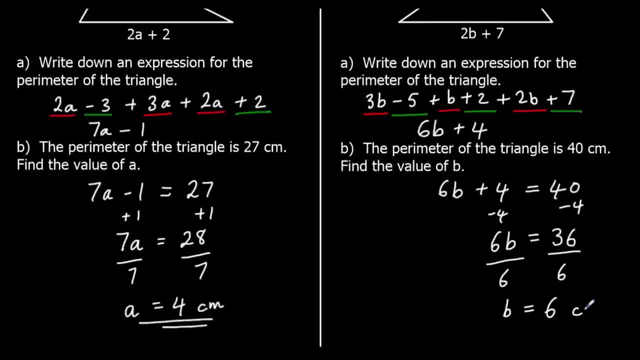 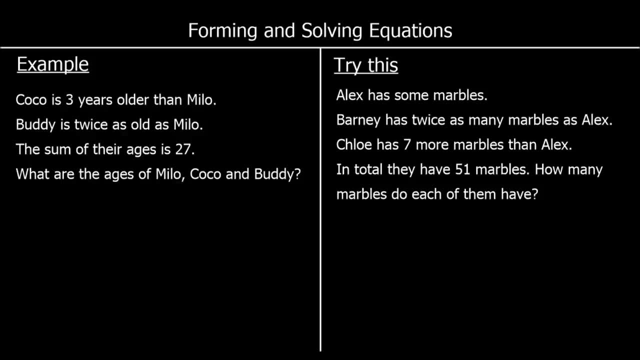 so b is 6 and i'll write centimeters again. okay, one more example. this time we're not looking at shapes, we are looking to form an equation from these statements. so the first one: coco is three years older than milo. buddy is twice as old. 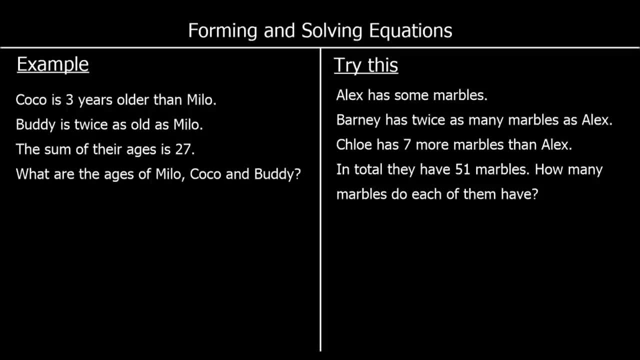 as milo, but he is twice as old as milo, but he is twice as old as milo, but he is twice as old as milo. the sum of their ages is 27. what are the ages of milo, coco and buddy? we're going to start solving this. we're going to start this question by calling something x. 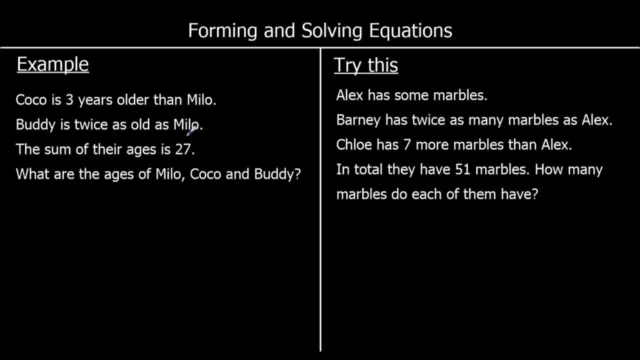 and milo is in both of these lines, so it'll be easiest if we call milo x. so if milo is x, milo is x years old. coco is three years older than milo and coco is three more. that's going to be x plus three. 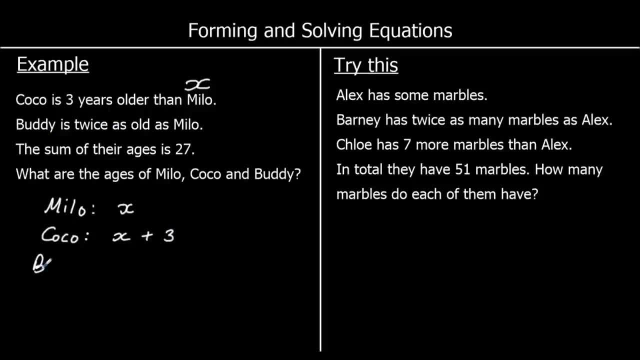 buddy is twice as old as milo, so milo is x. buddy is two times up, two times x is three years old. 2x in terms of X. we've got each of their ages and they, they sum. the sum of them is 27. so that means them all added up is equal to 27. so X plus X plus 3 plus 2x. 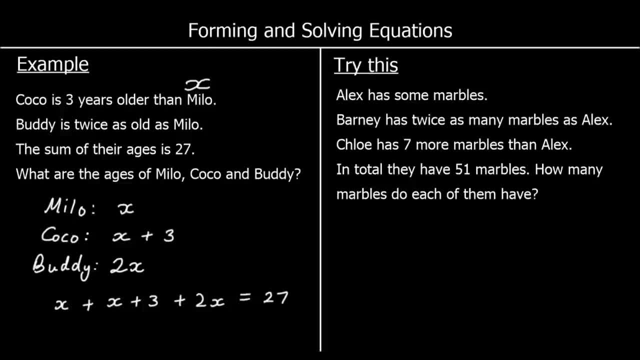 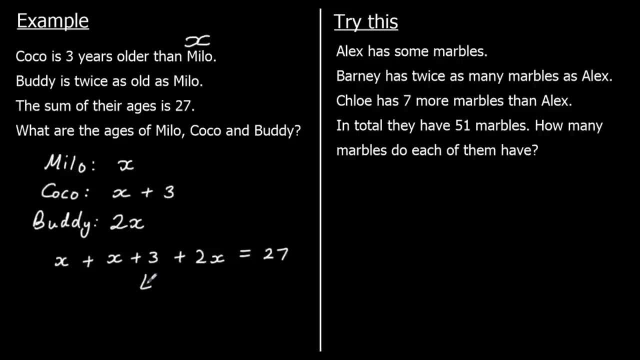 equals 27. so, simplifying this, we've got 1, 2, 3, 4, X's plus 3 equals 27. take 3 away from both sides, so we're solving now: 4x is 24 and to get X by itself, divide both. 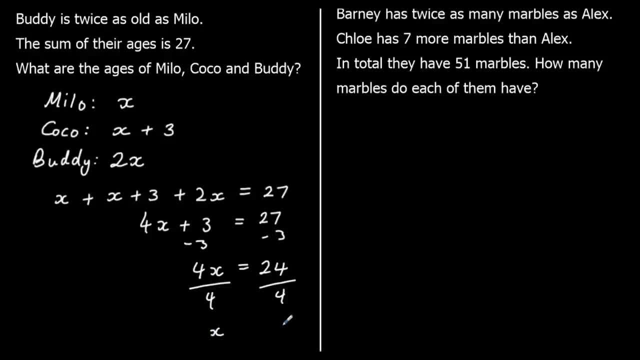 sides by 4, so 24 over 4 is 6, so X is 6. that means Milo is 6, Milo is 6, Coco is X plus 3, so 6 plus 3 is 9 and Buddy is 2x's, so 2x's. 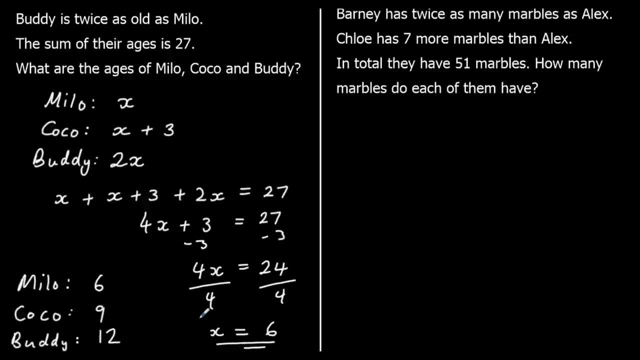 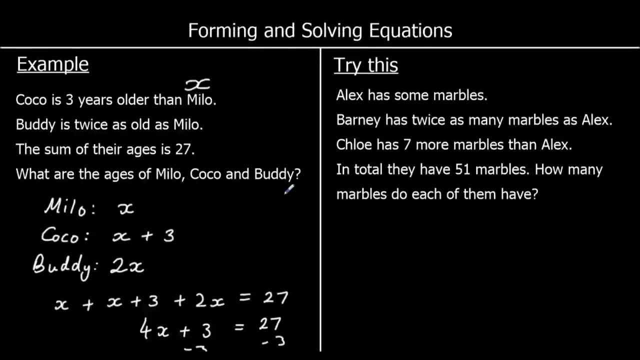 which is 12. okay, a question for you to try, so pause the video and give this one a go. the question says: Alex has some marbles. Barney has twice as many marbles as Alex. Chloe has seven more marbles than Alex. in total they are 51. how many marbles do each of them have? so let's call Alex X. Alex has X. 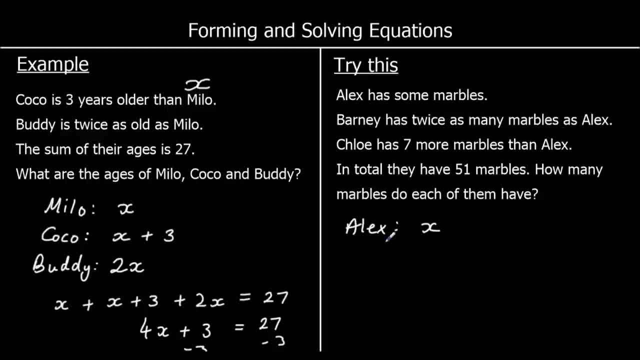 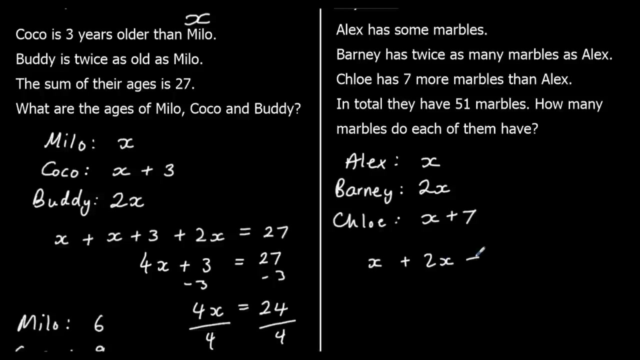 marbles. Barney has twice as many, which is 2x's, and Chloe has seven more than Alex, so seven more than X, which is x plus seven. so in total they are 51. so them all added up is equal to 51. so X plus 2x plus X plus 7 is equal to. 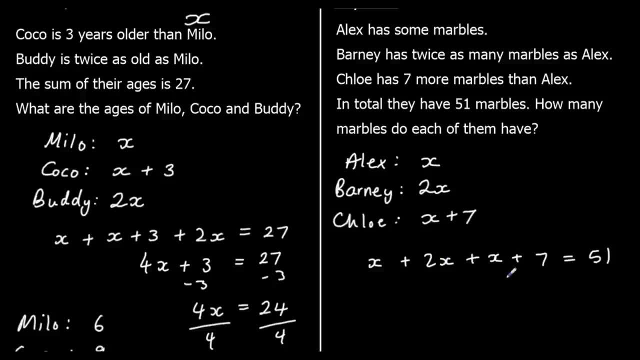 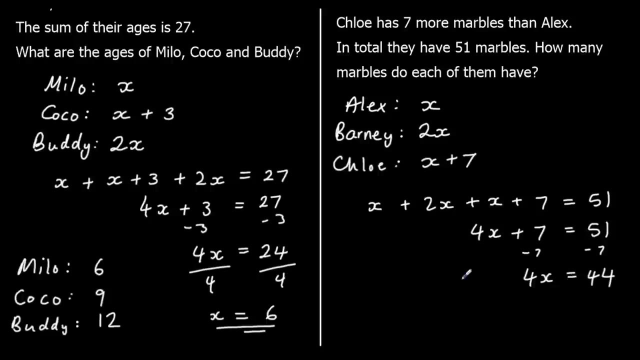 51. so 1, 2, 3, 4, X's plus 7 equals 51. so we'll subtract 7 from both sides, which leaves us with 4x equals 44. so divide both sides by 4 and that tells us X is. 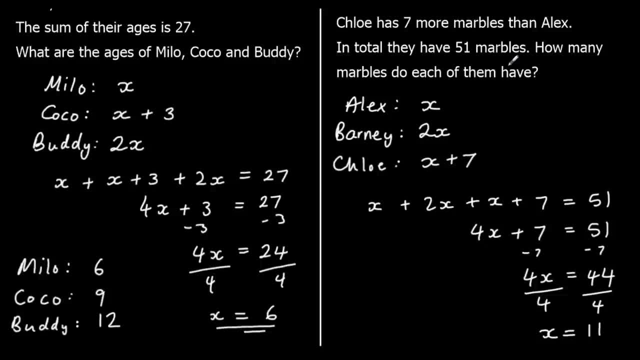 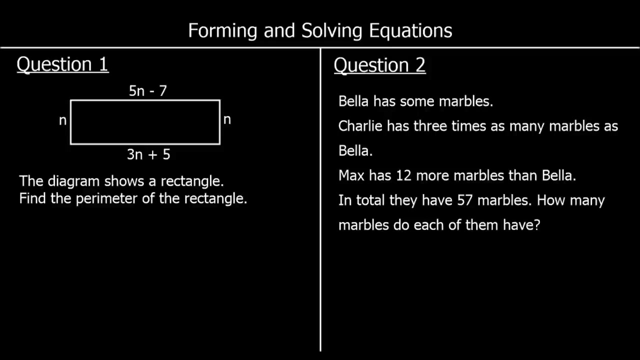 11. so how many to each of them have? Alex has X, which is 11, Barney has two X's, so 22, and Chloe has seven more than X, which is 18. so to finish up two questions. pause the video, give them a go and press play when you're ready for the answers question. 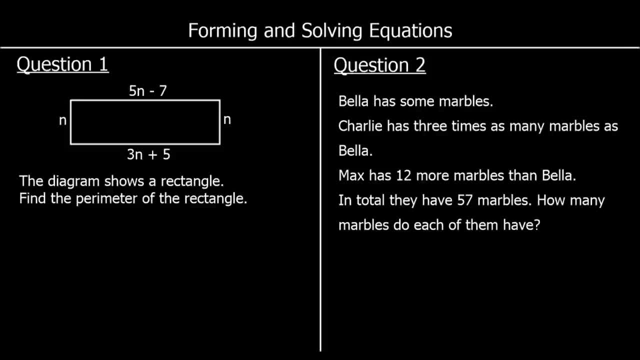 one. we have a rectangle and we need to find the perimeter of the rectangle. we're not given any length, but we do know that the opposite to length must be equal. so five and minus seven must be equal to 3n plus five, and we can solve this. 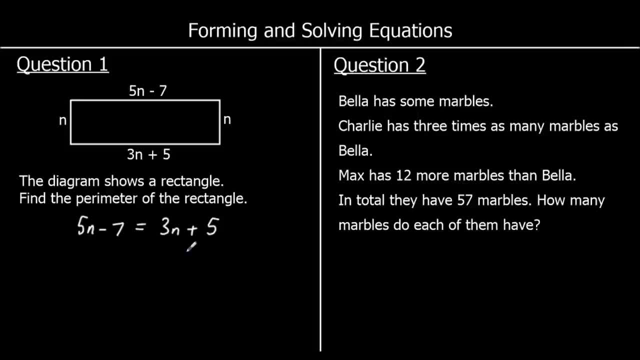 So take the smallest n away first. So we'll take 3n away from both sides, which will leave us with 2n minus 7 equals 5.. Then we can plus 7 to both sides, So 2n equals 12, and divide both sides by 2, which will tell us n is 6.. 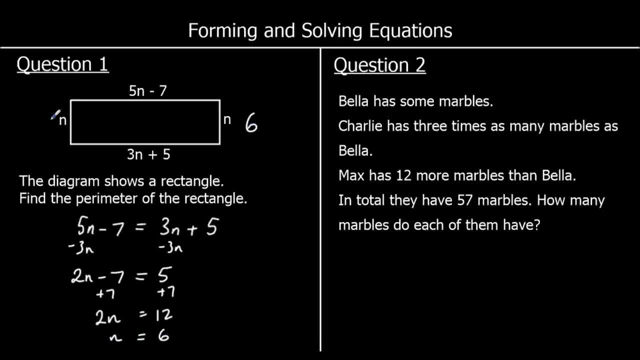 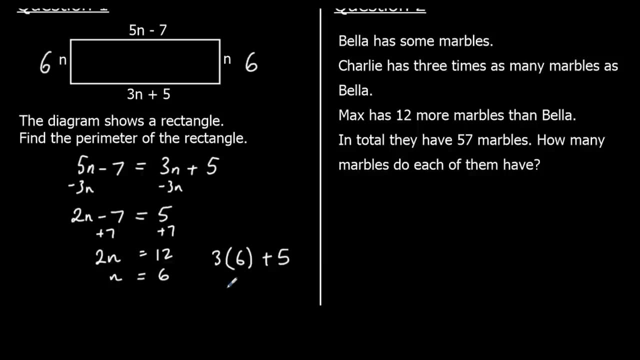 So we know that the two shorter sides are 6.. How big are the longer sides? So 3n. so 3 times 6 plus 5,, which is 18 plus 5,, which is 23.. So the two longer lengths should be 23.. And if we do 5 times 6 minus 7,,